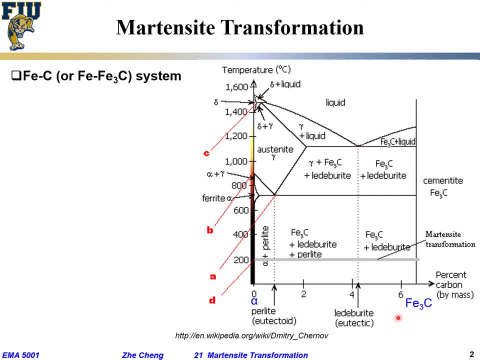 material based on steel are essentially based on this face diagram and you think, well, people use steel or iron almost everywhere, almost everywhere. remember earlier we mentioned the annual production of steel is iron and steel is almost 2 billion tons. 2 billion tons, which means two thousand million tons and all the other metal combined: aluminum, copper, titanium. 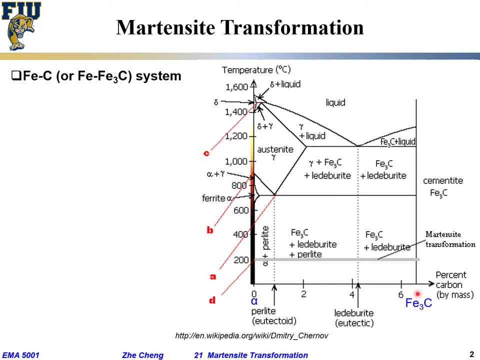 all the nickel, all those other metal combined. people are producing probably less than 50 million tons. one side is 2,000 million tons, one is 50 million. you see the difference between iron and steel, all the other metals combined for automobile. the majority are made of. 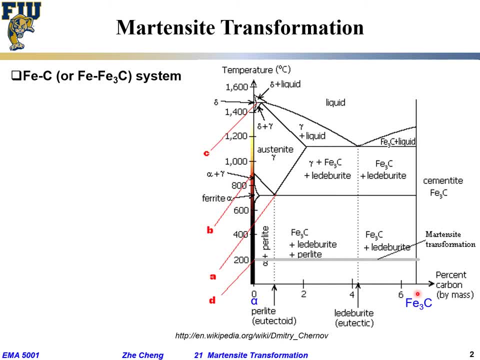 steel right for bridges, the construction material for bridges or for buildings. anyone using aluminum very little, very, very or negligible. anyone using titanium- completely negligible, right. so that's that's a fundamental reason- is okay, it's just everywhere. that's why people study this material so broadly. people use iron steel for almost everything: for knife- anyone see aluminum knife. 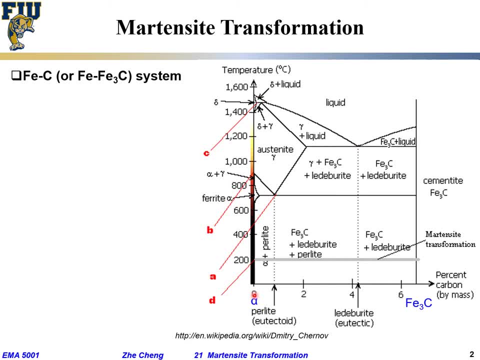 no titanium knife, no wood knife, steel, typically steel. maybe add some little bit element, stainless steel but steel. and then for any of the tool you go to home depot, all those tools, anyone making aluminum too no, titanium too no. why one for cost, one for mechanical property? they're not any better. 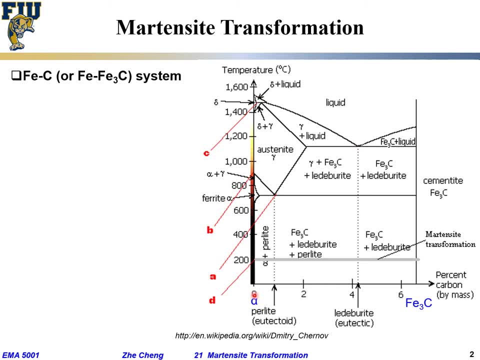 than steel too. okay. and any of the saw or two steel material, any of the saw. any aluminum saw saw blade: no. why too soft? any titanium saw: no, all of them are essentially steel, based from very soft steel, pure iron that people use for tongue twister, the, the pipe cleaner or for 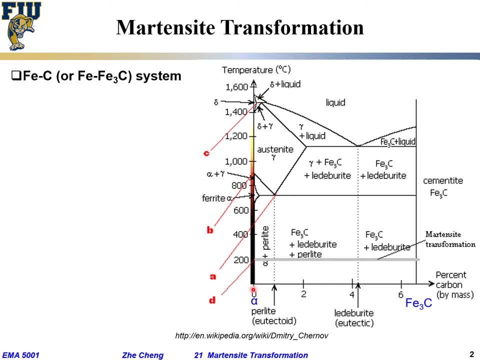 the types of material that goes into your typical tin can. actually people call it ting can, but actually it's almost a pure iron, not tin. okay, very soft iron to the very hard blade, the two steel, all those are made of iron. okay, your construction, all the building, the refrain, the 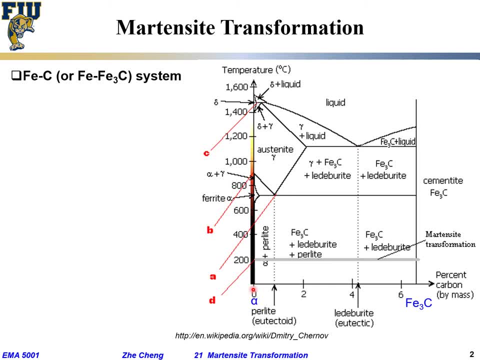 the, the nails, all the nails, all the screws. anyone see aluminum screw? why too soft? it's just too soft, okay, it doesn't. you screw it a few times the, you quickly lose the, the, the bite right. just for all these reasons people can, just by playing with the material composition, people can make the iron. 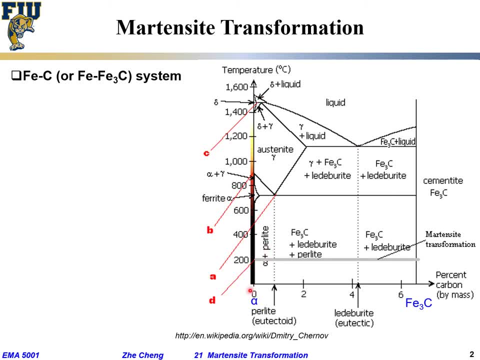 and one hand very, very soft for pipe cleaner which you can burn back and forth, or for the very hard knife right for knife saw blade, all those type of special for gear surface. anyone see aluminum gear quickly it would well. even if you make it quickly, it's expensive and even if you make it. 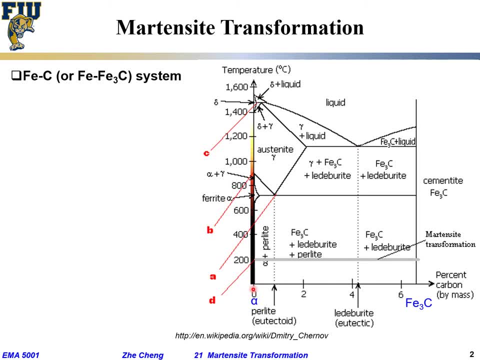 quickly, well off. people always make steel, some type of steel gear, right. so for all these reasons that people can change the carbon concentration change, adding a little bit of alloy element, people can make the steel almost a broad changing property and use it very widely. so we are looking. 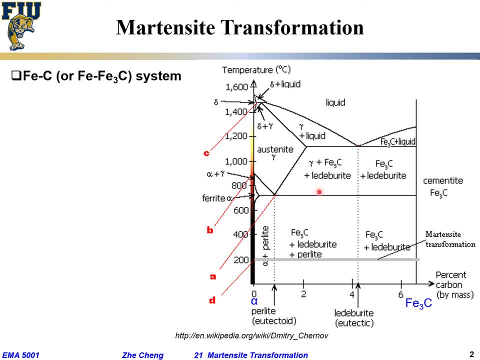 at the phase diagram. very important again, it's the most important phase diagram. again, at higher temperature we have what phase liquid right, which means uniform liquid above this so-called liquidus line, and then near the pure iron side, at close to 1500 degrees c, we have the melting point for 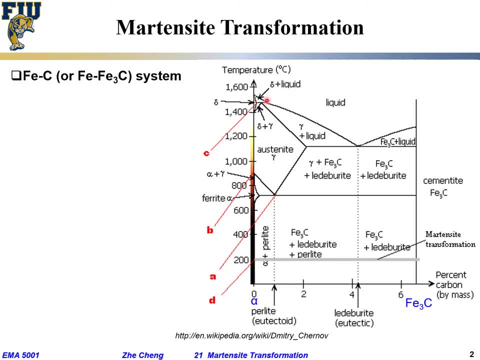 almost the pure iron, okay. and then we have a few phases, a single phase and two phase region. one is this so-called we label and see is actually so-called. the delta phase. okay, high temperature, bcc iron. and then we have a wide region which people call. 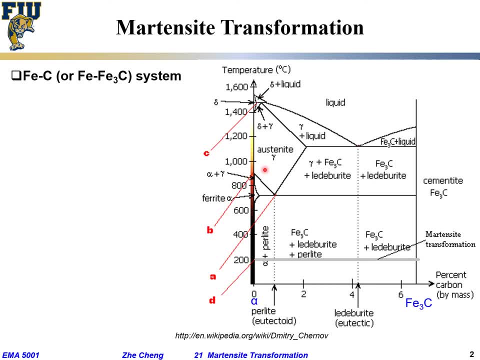 austenite, right austenite, that is, the so-called fcc iron, the iron item arranged as a phase centered cubic structure. okay, and then a little bit lower, we have the so-called the fire right alpha, which is bcc ion, and on the other side we have the cementite. 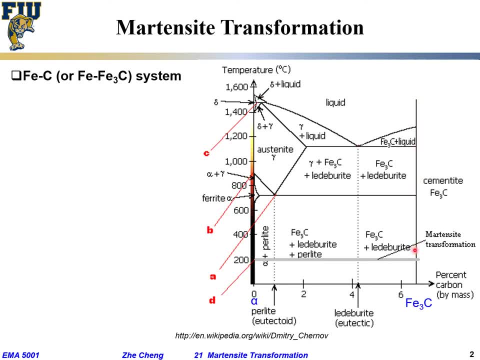 cementite, which is essentially a- we call it line compound. very little deviation in the composition. a so-called line compound cementite. iron 3c. okay, and then between single phase and the, between two single phase regions. there are always two phase regions, For example between liquid and austenite, between liquid on the top and austenite or gamma phase on the left. we have two phase region right, And also between liquid and the lime which is our cementite. we also have the iron 3C plus liquid. That's also a two phase region. 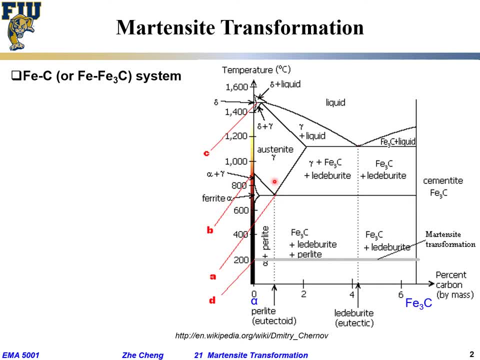 Similarly, a little bit lower between austenite gamma and that in the lime Fe3, we have the two phase region. okay. Of course people give it a different name, but essentially it's gamma plus cementite. okay. 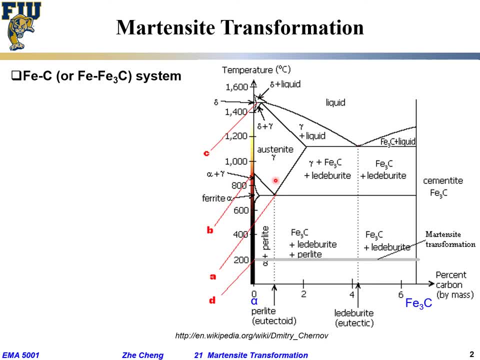 And then, if we keep going down the temperature between gamma and alpha, we have this two phase region between gamma and alpha. We have this. one would be the two phase region of gamma plus alpha right. And then, of course, if we keep lowering down the temperature at here where I'm pointing, which is on one side, left side is alpha, on the right side is cementite, okay, 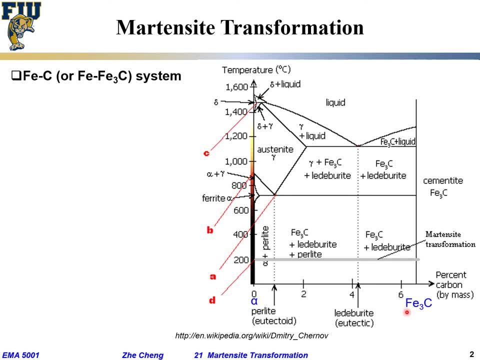 On the left side is alpha, on the right side is cementite. In between, from here all the way to here, From left all the way to right, as long as temperature is low, we have two phase region, Essentially what? Alpha plus iron 3C. 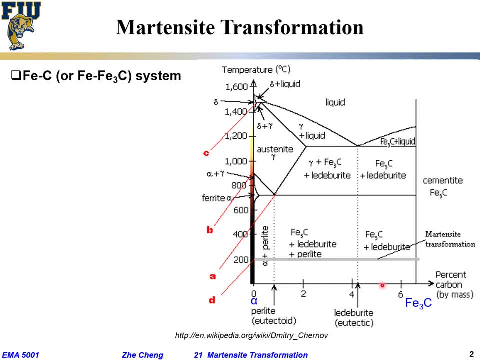 That's a two phase region. okay, Of course, in this phase diagram a little bit complex. people call it pearlite and some other name, but essentially all those are still alpha plus cementite, which is iron 3 carbon. 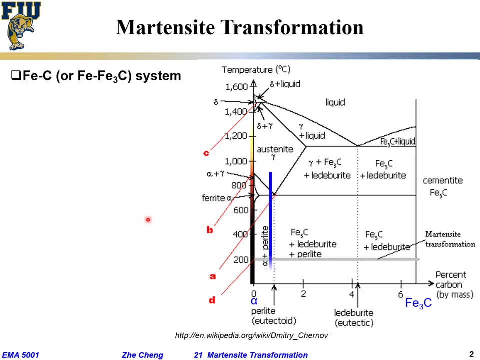 So for such a system, if We look at a specific composition, that okay, as we illustrate it in this blue arrow, this blue arrow were cooling from what? austenite gamma phase, single phase into the two phase region. okay, 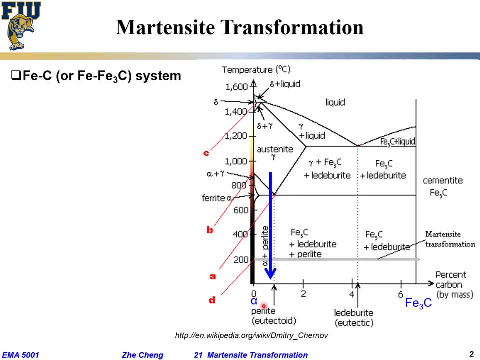 Under equilibrium condition. what should happen If we could do very, very slowly, we would get a one phase is alpha on the left, the other phase would be the cementite Fe3C on the right. but what people find is, if people do this quickly, like an iron smith he would put his red. 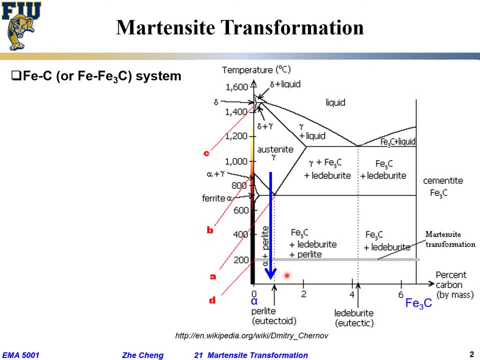 hot iron deep into oil or sometimes even water. people find with extremely rapid cooling and people find the extremely rapid transformation, rapid transformation of the high temperature phase, the gamma phase austenite into the fine hard structure. what type of structure it's actually? 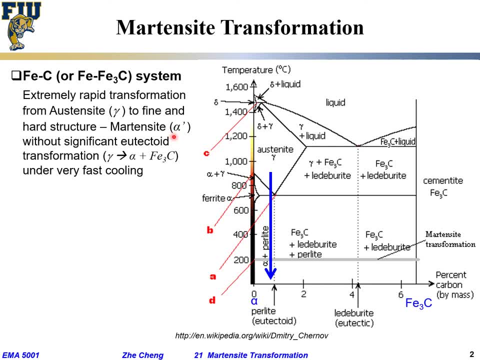 people call it alpha ion, alpha prime. it's like a BCC, similar but not exact. people call it a martensite without significant eutectoid transformation, which is it doesn't really go through the equilibrium reaction from gamma to alpha plus Fe3C cementite under fast cooling. 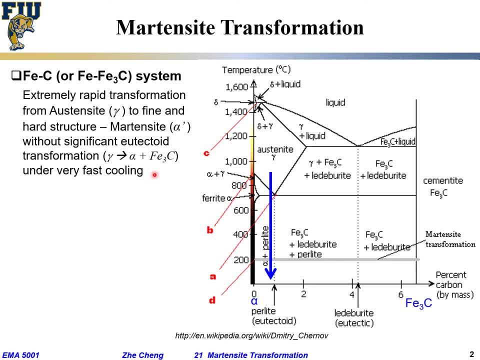 this type of phenomena. people call it martensite transformation. okay, and what we are going to talk about is it's a transformation into a so-called metastable. metastable means it's not exactly the alpha prime or the martensite. the alpha prime or the martensite, it's not the most stable. 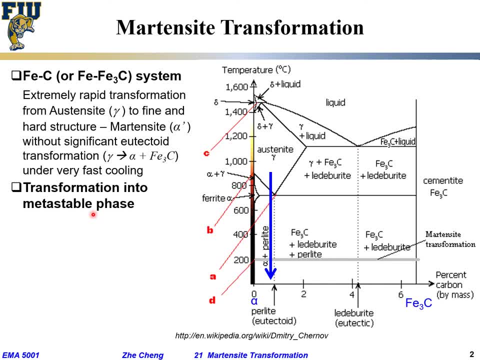 phase. under that condition, it's not the lowest energy state, but because we are doing this in a fast or slow process- fast, actually, very, very fast process- it end up in this so-called metastable state. this is a martensite transformation and if we 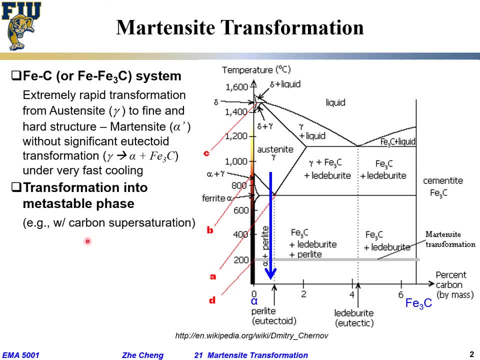 want to talk about a little more. this martensite phase would have read carbon supersaturation, this so-called alpha prime phase. it's a single phase, but the carbon is oversaturated, which means the carbon concentration within this alpha prime is higher than it actually can handle. but it just